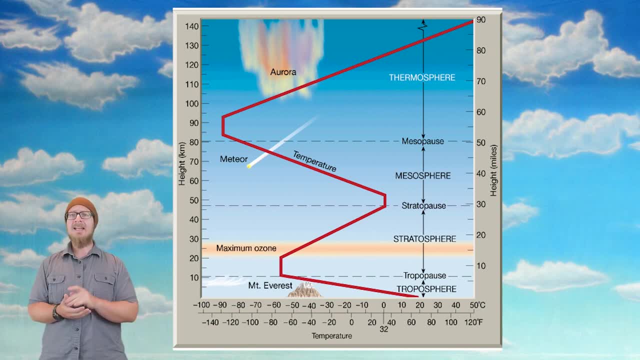 temperature as you move up through the layers. At each inflection point or where there's a change in the direction of a temperature change, we call that a pause. There are four layers to our atmosphere and the first is the troposphere. Moving up from there, we get the stratosphere, which contains the ozone layer, then the mesosphere, where entering meteorites tend to burn up, and then the thermosphere, which contains our ionosphere. that protects us from the battering of charged particles from the sun. We call that solar wind. 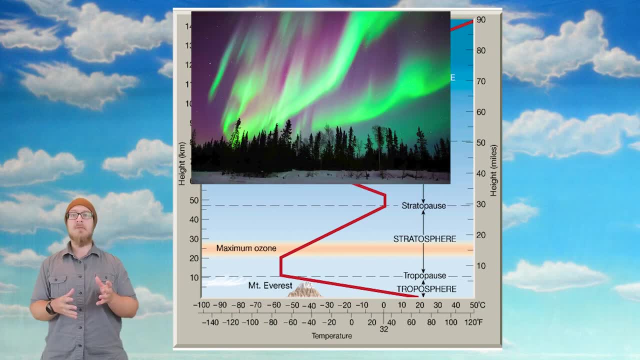 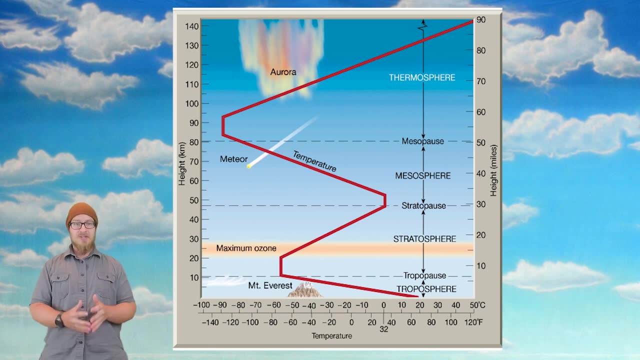 and the interaction between solar wind and our ionosphere is what well creates the aurora lights. Let's begin our discussion with the troposphere, as this is where just about everything that matters to us occurs. The troposphere is where we get weather and I. 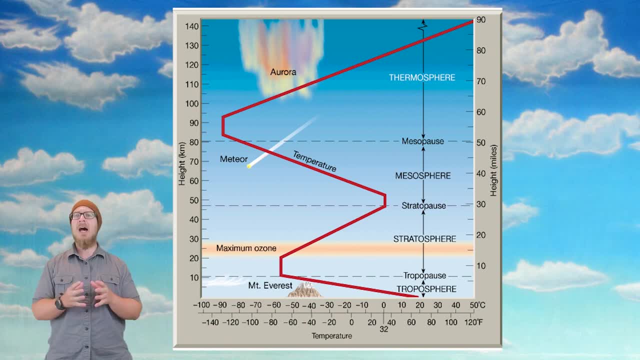 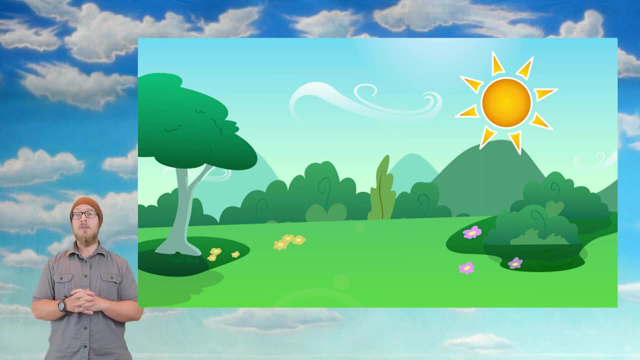 thought it might be useful to do a brief discussion on why it rains. It begins with the sun that sends light rays towards our planet. Those light rays are absorbed by the ground and re-emitted up as thermal radiation or heat. I want to note here that we don't actually get any appreciable heat from the sun, like at all, I mean. 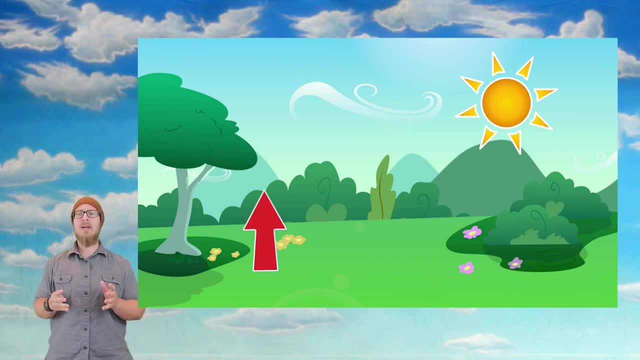 the sun is hot, but we are very far away, so we don't actually get much heat from the sun. The thing that warms the troposphere ends up being the ground that absorbs the sunlight energy and radiates it back up as heat. So while the ground is heating the air above it, the sun's energy is also causing 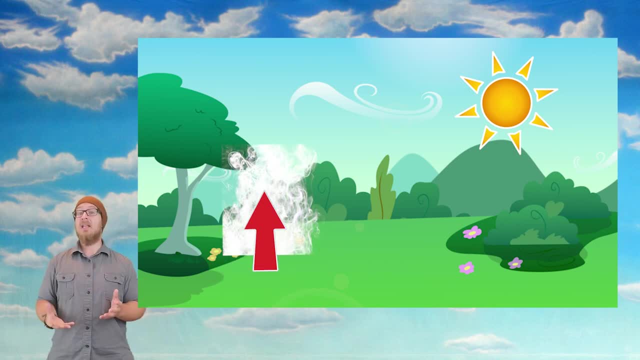 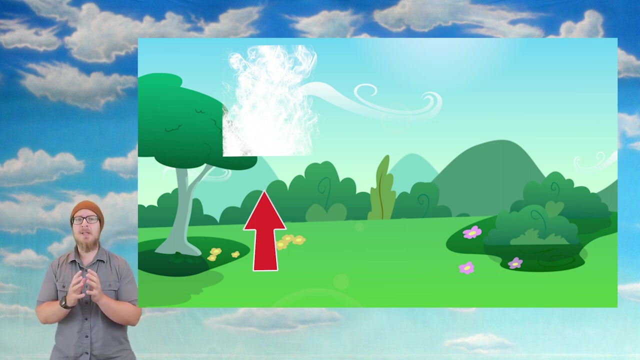 water to evaporate. The warm air is less dense and begins to rise, well, as does the water vapor. We call this an updraft. Eventually it gets farther from the ground and cools off. This is where the water vapor part becomes important. See, warm air is very good at like holding onto water, which is 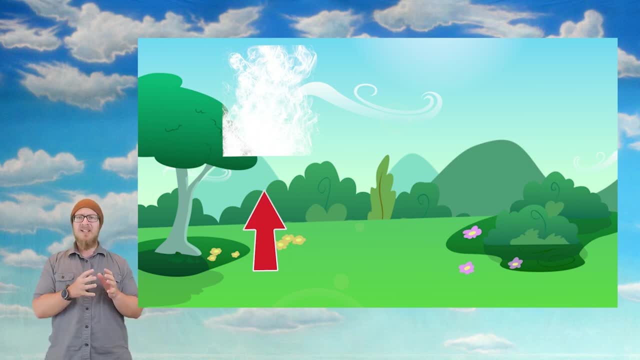 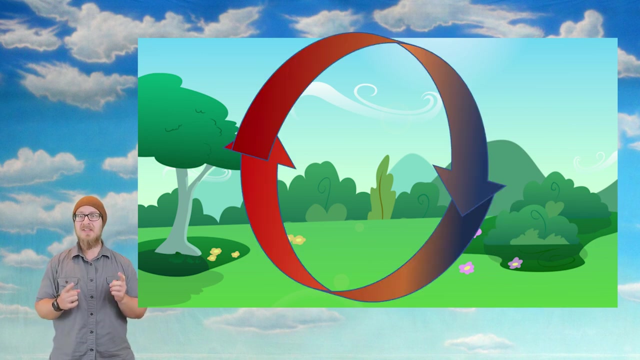 why it tends to be humid during the summer, Cold air not so much So. when the water vapor and cold air get that high, the water condenses into clouds. As water droplets grow larger and heavier, gravity pulls them down. That's rain. Eventually, the cooler air will fall too. We call that a downdraft. Wait, is this what? 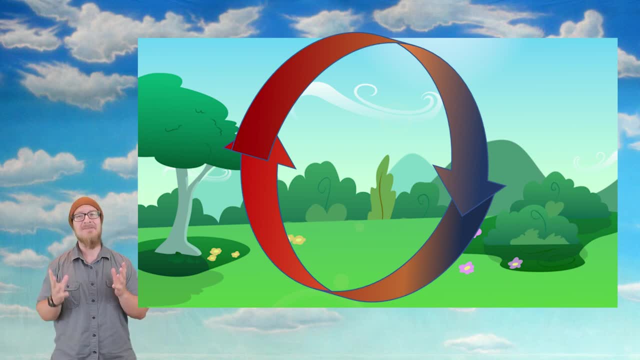 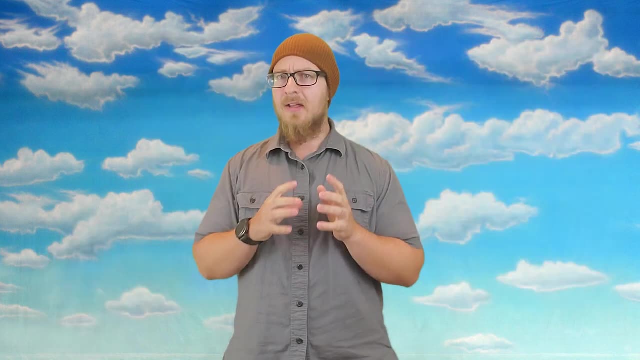 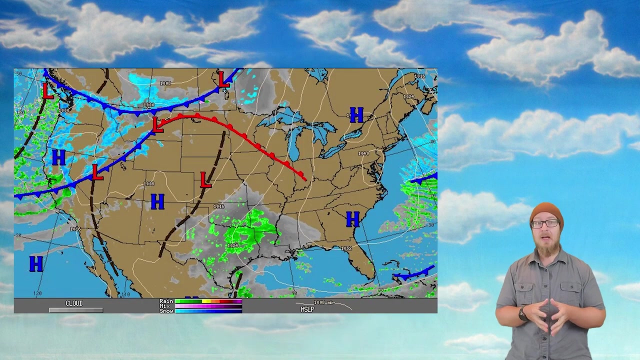 I think it is. Oh look, it's one of those convection cycles we've learned about. Oh, convection cycles are so very exciting. That said, the air in the atmosphere isn't particularly homogenous. There are areas where the air is colder and a bit denser. We call those high pressure systems. 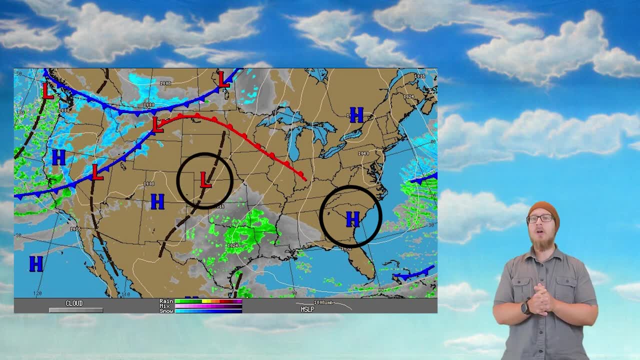 And there's areas where the air is warmer and less dense. We call those low pressure systems. Now let's say you get a low pressure system and a high pressure system interacting. The separation between those air masses is called a front. That's what those 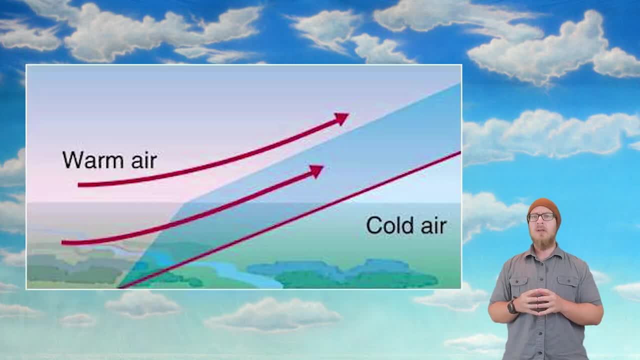 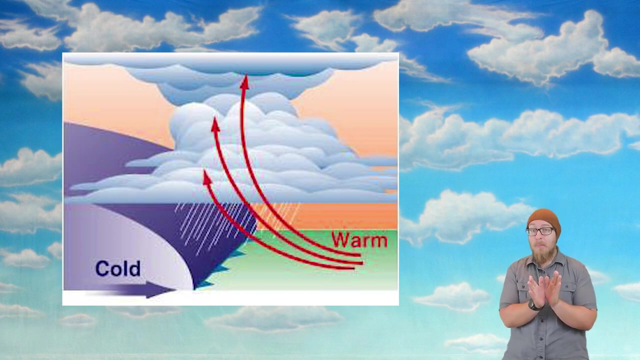 lines in the weather forecast are trying to show you. If a low pressure system is pushing into a high pressure system, the less dense warm air will float gently above, will eventually cool down and cause rain. If a high pressure system is pushing into a low pressure system, the cold. 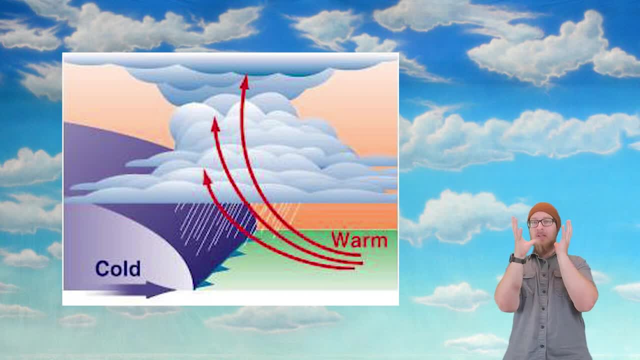 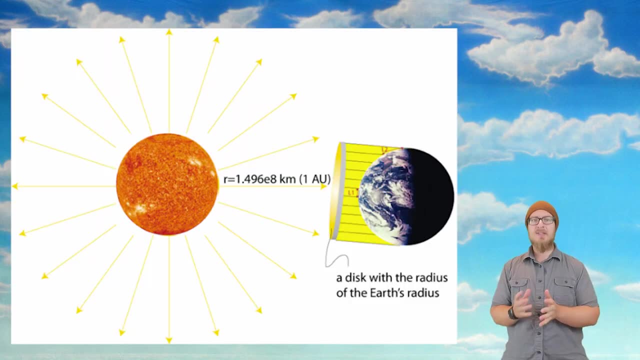 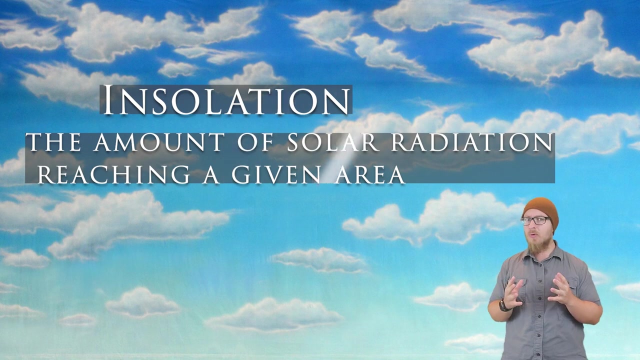 dense air acts much like a battering ram, forcing the warm air upwards. This results in storms. Now, the reason the air isn't so homogenous is because the sun shines a bit differently depending on where you are in the planet. Insolation is the amount of solar radiation reaching a given area. 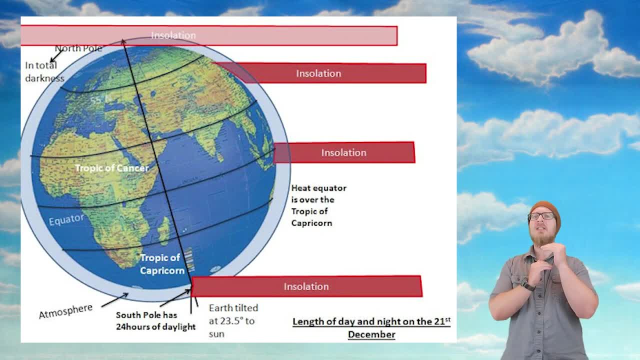 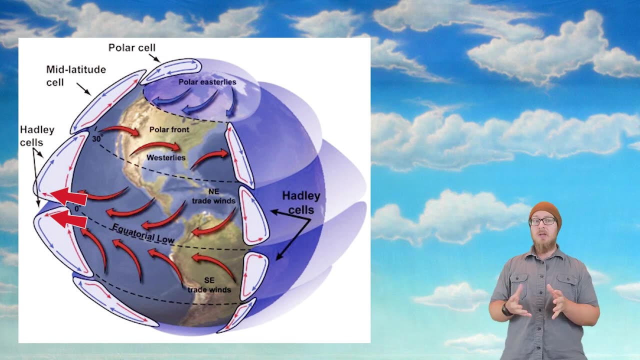 occurs at the equator, and the insulation decreases as you go farther towards the poles. This difference in insulation is what produces global wind patterns. Notice how the equator has two updraft systems. This is because the equator gets the most sunlight. This is the same reason why it rains more near the. 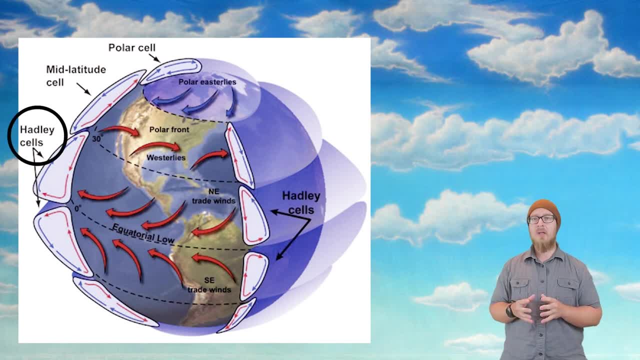 equator. Now, if you look at the diagram, you'll notice that we named the giant convection cycles happening near the equator, the Hadley cells, And you'll note that the downdraft system from those Hadley cells where the dry air falls, 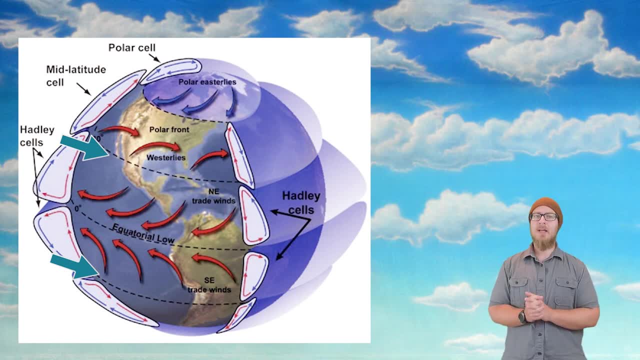 matches the general location of deserts in our planet. The mid-latitude cells, just above the Hadley cells in the north or just below in the southern hemisphere. those are the cells that contribute to the wind patterns. we see where my students and I are located in Chicago. The polar cells, which are at the 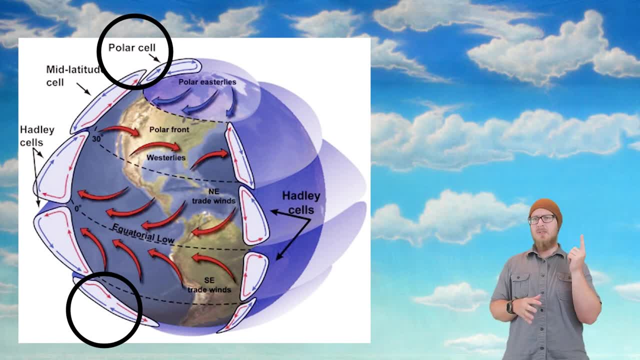 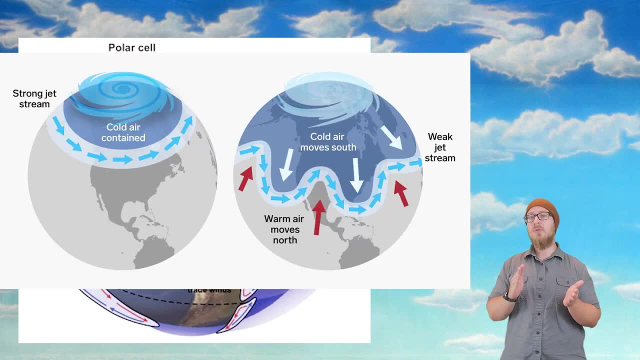 farthest- north or south usually- are limited to those. They kind of spin in a vortex all the way around, kind of staying more or less limited to themselves, But sometimes they do dip down, causing really cold temperatures in northern Europe and the northern United. 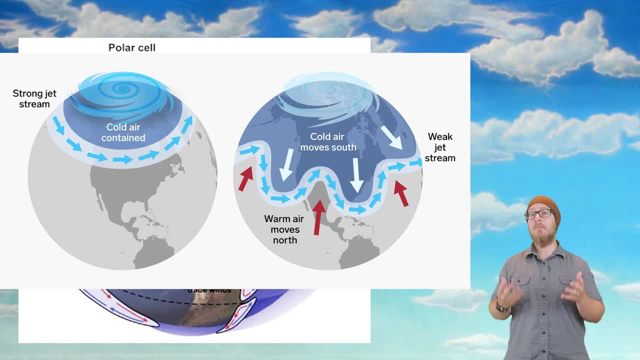 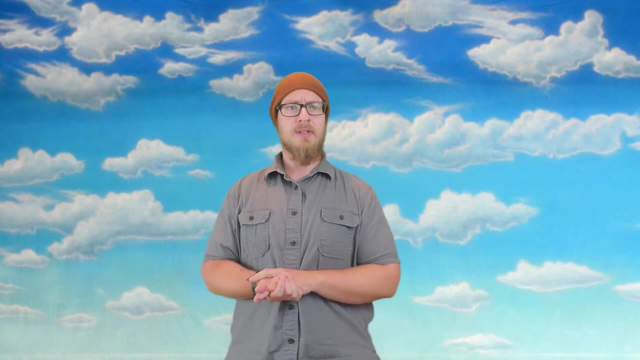 States area in a phenomena the weather people have been calling the polar vortex. But wind doesn't just move in one direction, like these convection cycles would lead you to believe. Take a look at the winds that the diagram has labeled here: The westerlies. 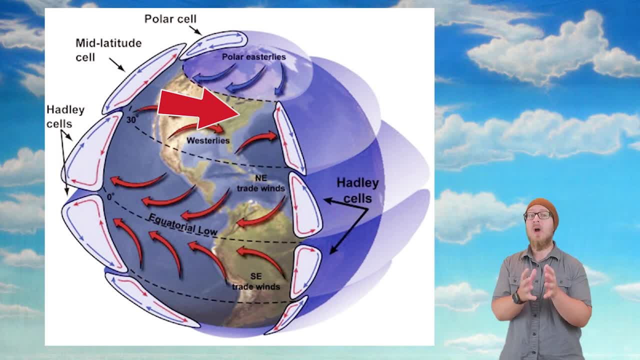 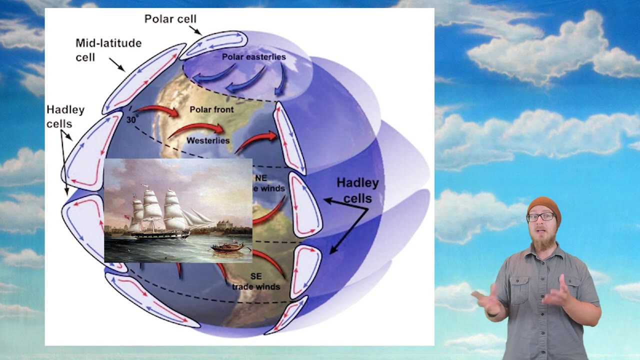 are so unnamed because they originate from the west and the easterlies originate from the east. The trade winds are just fancy names for the easterlies we see near the equator, and they're called the trade winds because those are the winds that push the sails of the old trade ships to navigate across the ocean. But why do the 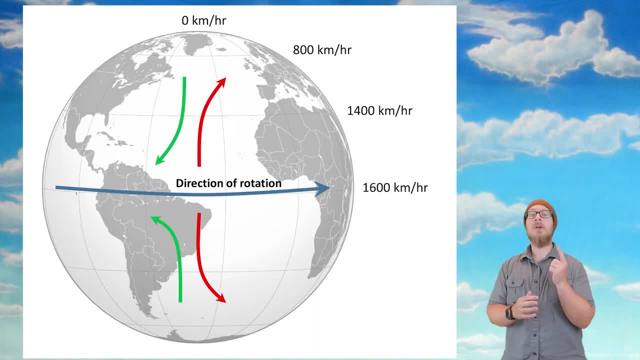 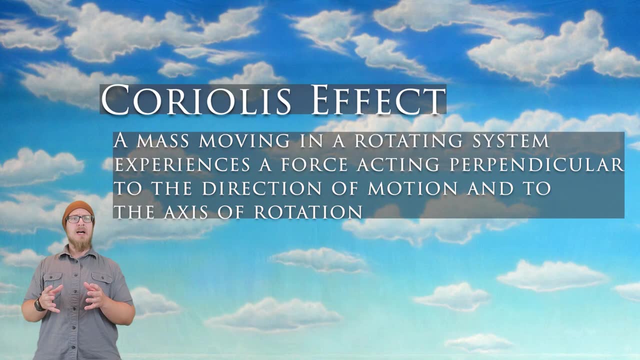 winds deflect like this. Well, you see, the earth spins and as it spins, wind gets deflected due to the Coriolis effect, An effect whereby a mass moving in a rotating system experiences a force, the Coriolis force, acting perpendicular to the direction of motion and axis of 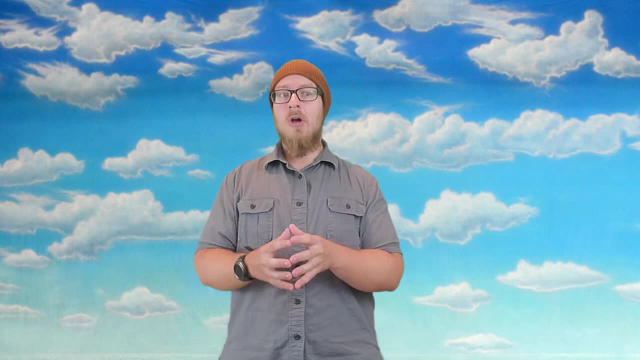 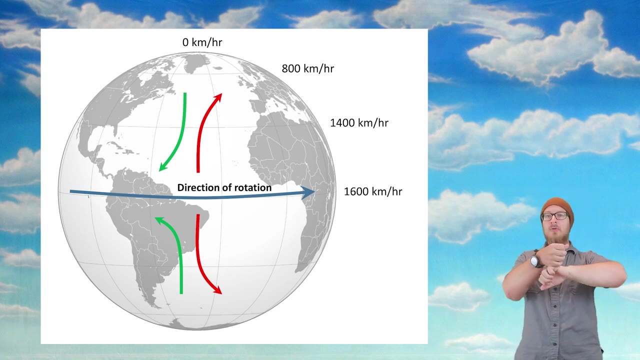 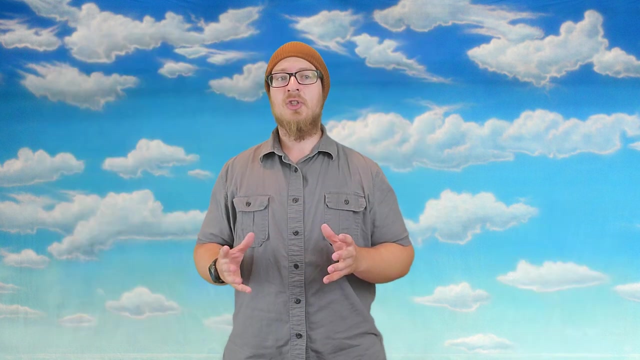 rotation. Now, those are very technical words. All it means is that if you begin at the equator and travel north, objects veer to the right. If you travel south from the equator, things tend to veer to the left. This difference in insulation- 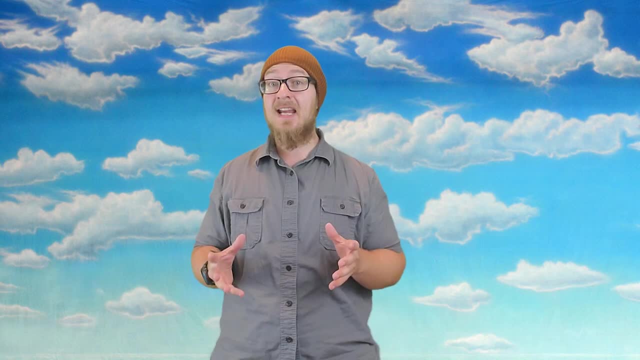 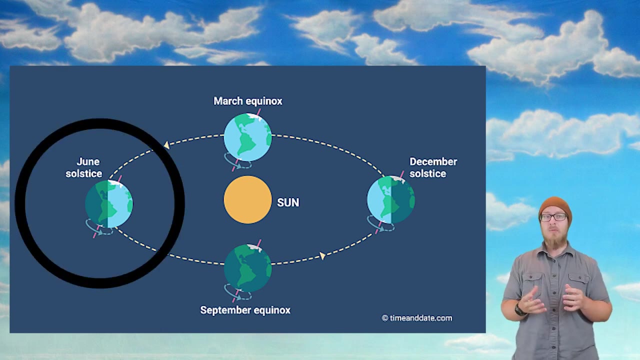 doesn't just produce the wind patterns, it also dictates our seasons. The Earth is on a tilt And because of this tilt, the Northern Hemisphere gets more direct sunlight during our summer and the Northern Hemisphere gets less direct sunlight during our winter. You'll notice this. 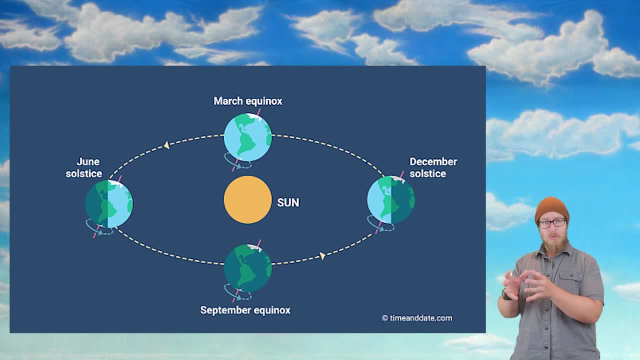 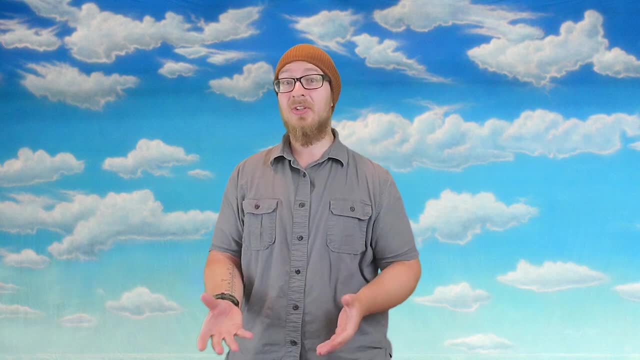 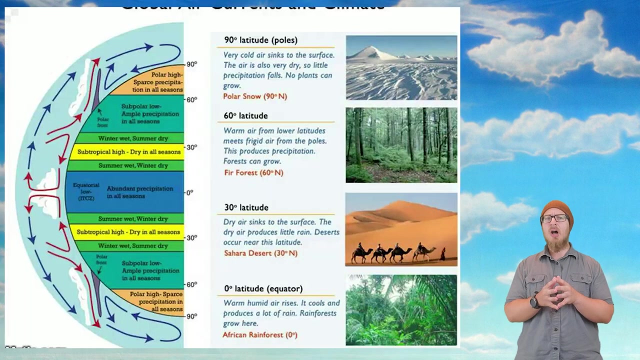 is the opposite in the Southern Hemisphere. When it's winter up in the northern half of the planet, it's summer in the Southern Hemisphere. So yeah, the Australians celebrate the winter holidays at the beach, Ready for more sun. stuff The insulation, in combination with those wind patterns. 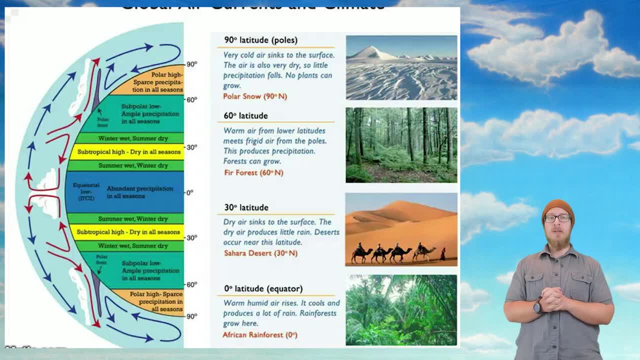 is what dictates climate on Earth. It is warm and rainy at the equator because of the updrafts and direct sunlight. It is hot and dry at the deserts because the 30-degree latitude areas get a good amount of sunlight but experience the downdraft of dry air from those Hadley cells. The 60-degree latitude landscape gets a good amount of sunlight, but experience the downdraft of dry air from those Hadley cells. The 60-degree latitude landscape gets a good amount of sunlight, but experience the downdraft of dry air from those Hadley cells. The 60-degree latitude landscape gets a good amount of sunlight. 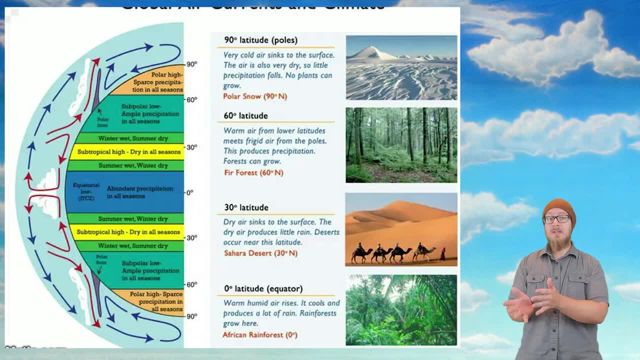 see temperature and seasonal climates because of the seasons and experience the updraft of the mid-latitude cells. but because there is less sunlight it's not quite as warm or rainy as it is at the equator. The far northern latitudes are cold because they don't get much direct sunlight at. 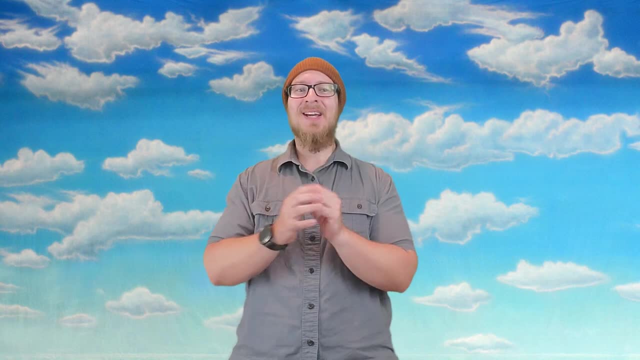 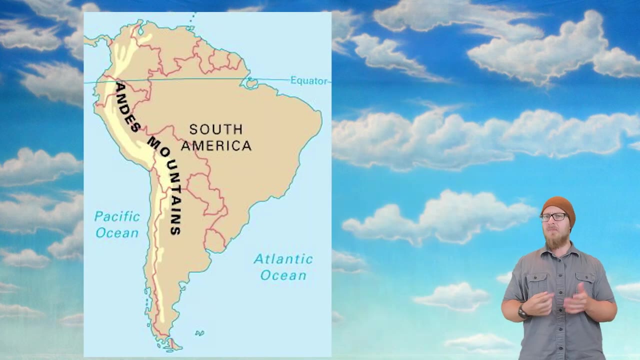 all. But wait, there's more. Just the amount of sunlight isn't enough to explain some climates. Look here, These are the Andes. It's a mountain range on the western coast of South America. Let's move up to the Colombian part of the Andes and look at Mount Louise. If you look at the 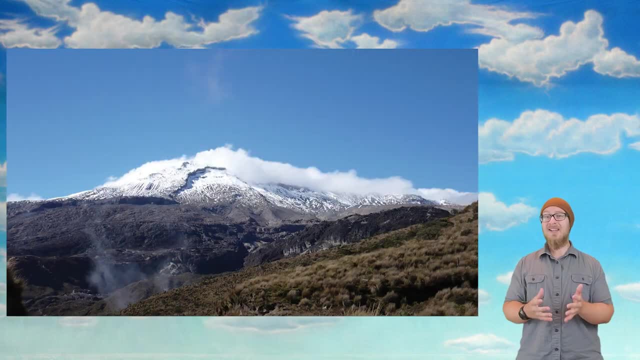 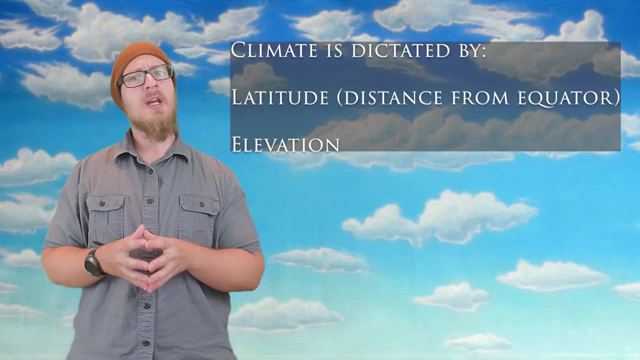 latitude. you'd think it's hot there, but look, It's ice. The higher in elevation you are, the colder the climate is going to be. So an area's climate is really dictated by two things: The amount of sunlight an area experiences and the amount of sunlight an area experiences. So if you 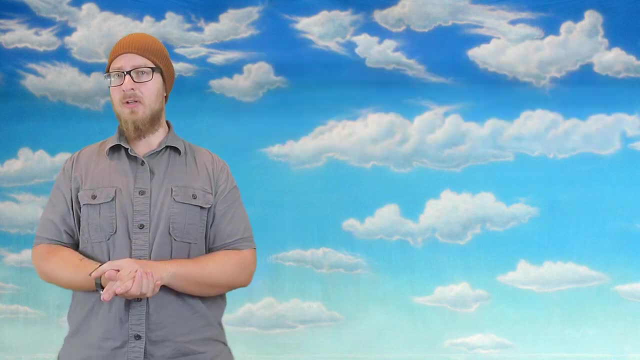 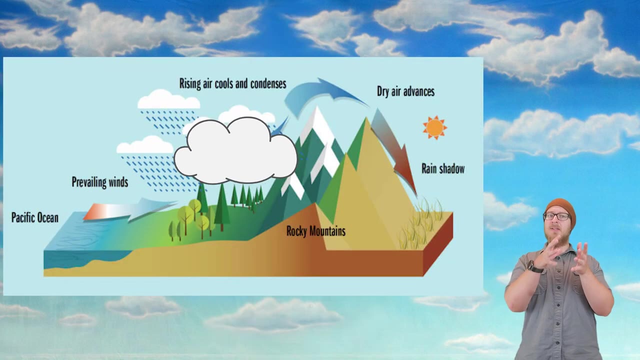 look here. you'd think it's hot there, but look, It's ice. The amount of sunlight an area experiences and the amount of sunlight an area experiences and the geographical features, like elevation Mountains, by the way, can also affect climate. Remember how rain is formed, by air masses being pushed up. Well, mountains can cause this too. In the mountains we see this rain shadow effect: Wind blows air up a mountain and the increase in elevation causes the water to precipitate out. By the time the air makes it to the other side of the mountains, it's lost all of its moisture. 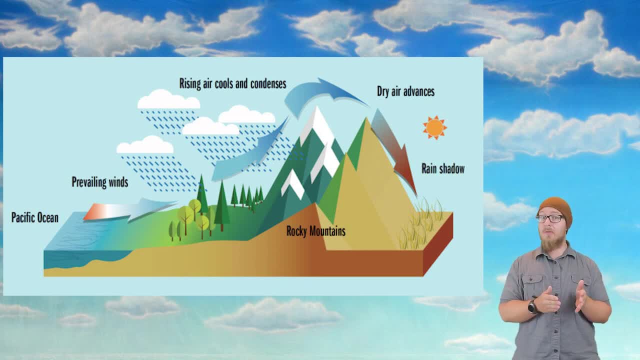 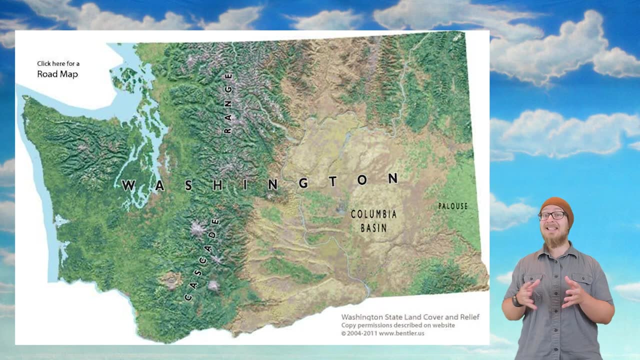 This area on the far side of a mountain is called the rain shadow because the mountains are shadowing the area from the rain. In Washington, the Cascade Mountains cause a rain shadow that causes the eastern side of the state to be kind of dry and the western side of the state to be. 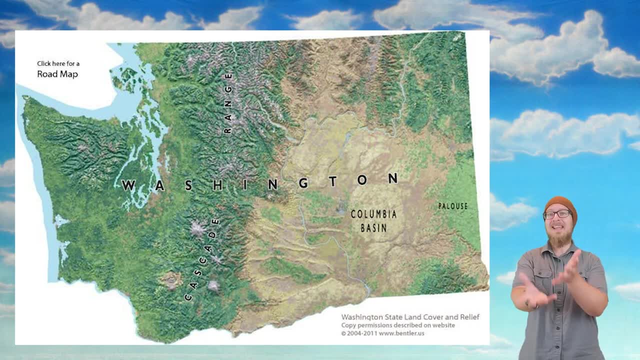 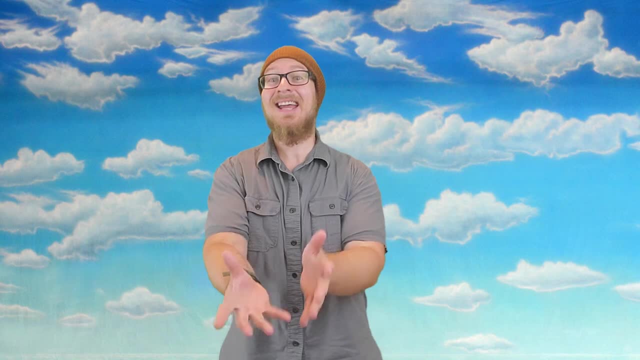 well rainy. That's also why it's raining in Seattle all the time, which explains a lot about Grey's Anatomy All this time, and we were only still in the troposphere, we were only still in the stratosphere. So I think it's time to move up in the stratosphere, And the stratosphere contains. 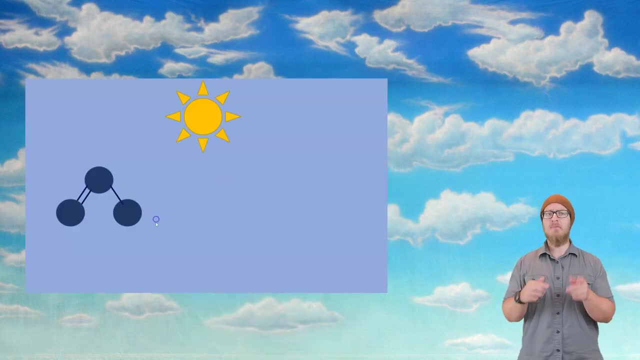 the ozone layer. Now ozone is this molecule I've got in blue here that is composed of three oxygen atoms. Now, ozone in the troposphere is generally bad. It's a lung irritant and causes breathing issues. But ozone in the stratosphere is great. It protects us from the sun's harmful rays. 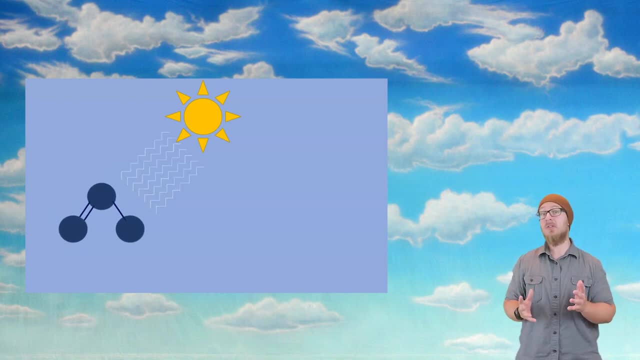 Now we already know that the sun shines light and it looks white to us. But white light is just what you get when you combine all the colors of the visible spectrum. But hidden in this light is a light we can't see, the ultraviolet. Now most light will pass through. 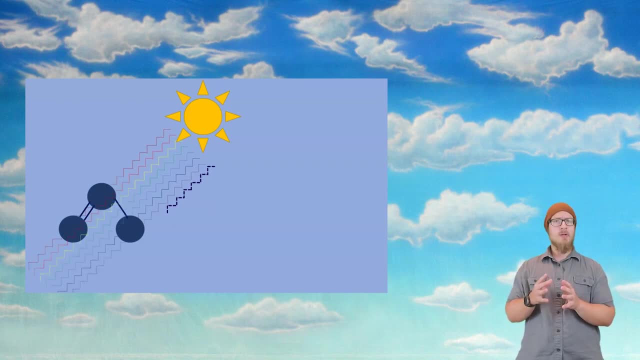 the stratosphere or less undisturbed. But notice what happens to our UV light. It seems to stop. Well, let's isolate this and see what happens. When UV light hits the ozone, the energy gets absorbed and causes a bond to break. This breaks off one free radical oxygen. 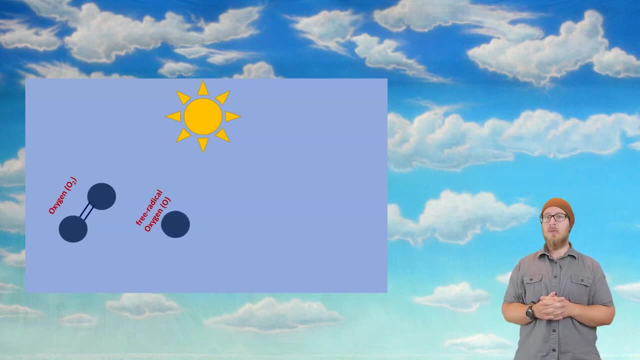 atom away from the well diatomic oxygen molecule. After some time the single oxygen atom will meet back up with the oxygen molecule and reform into ozone. This continuous absorption of ultraviolet and reformation of ozone protects us from most of the UV, But some still gets. 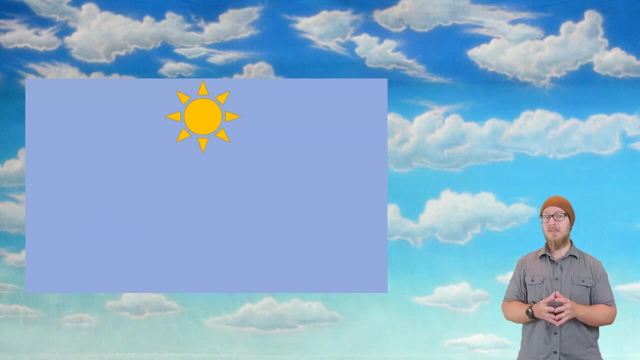 through Well for the UV that does get through well. if it were to hit the DNA in our cells, it would cause bonds to break and damage our DNA. Now, our body has ways to repair damaged DNA, but if it happens too often, your body might make a mistake, which can lead to cancer. 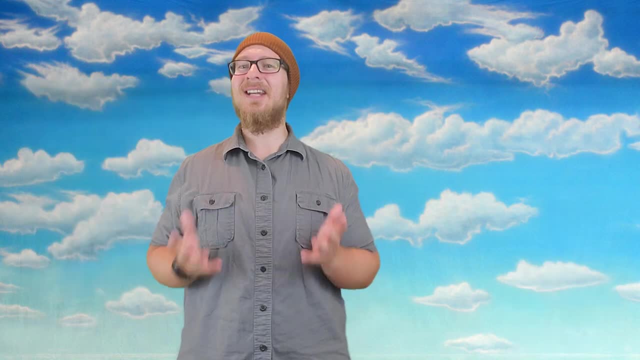 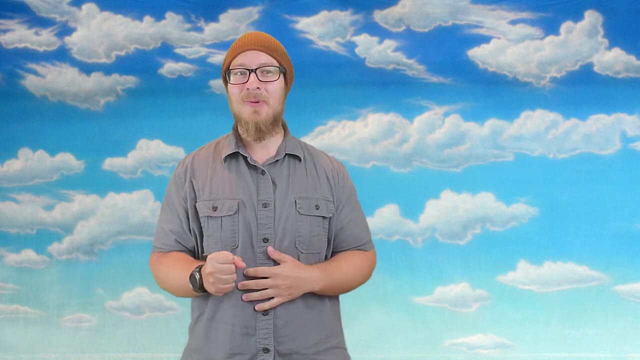 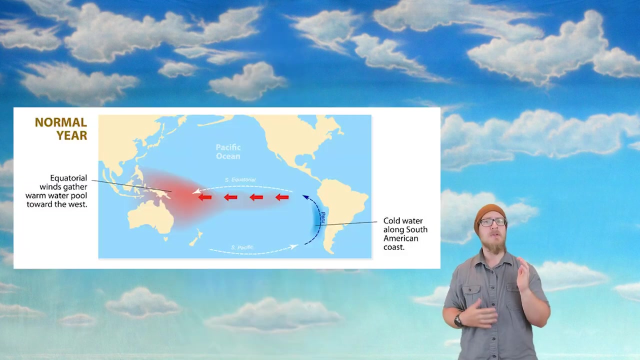 So, even though we have an ozone layer, wear your sunscreen anyway. The other parts of the atmosphere are beyond the scope of this class, so it's back down to the troposphere. We go for one last topic. This is a very unique interaction between the hydrosphere and the 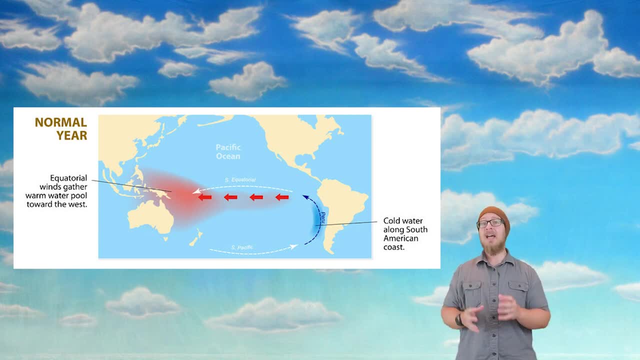 atmosphere in the Pacific Ocean. The El Nino Southern Oscillation is a pattern of weather changes that we observe in the Southern Pacific Ocean. Let's look at what the normal conditions in the Pacific Ocean are, the ones that occur the majority of the time Along the Southern Pacific. 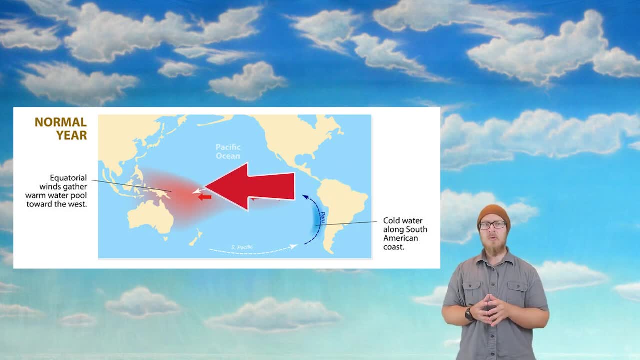 the winds blow away from South America and towards the Southeast Asia and Australia side. As these winds blow, they drag the top layers of water in the ocean to the other side, which causes a buildup of warm water on the western edge of the Pacific Ocean. This creates a warm and rainy 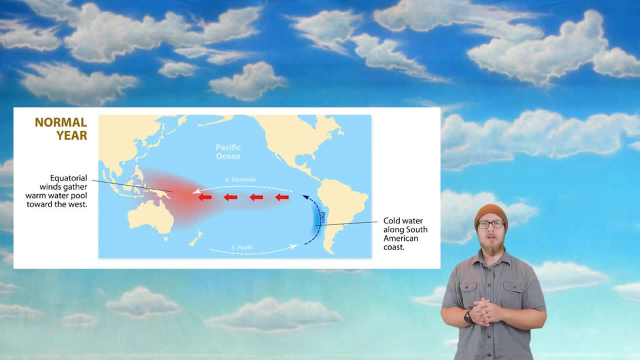 climate in Southeast Asia and Australia. Along the South American coast, the warm water that got blown away is replaced by cold water from deeper in the ocean in a process called upwelling. This water from deeper in the ocean is very rich in nutrients and produces a vibrant fishing. 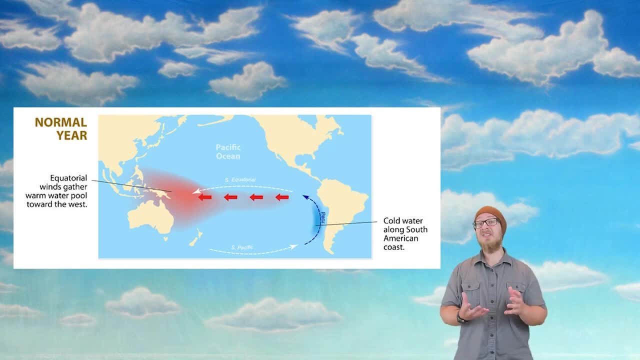 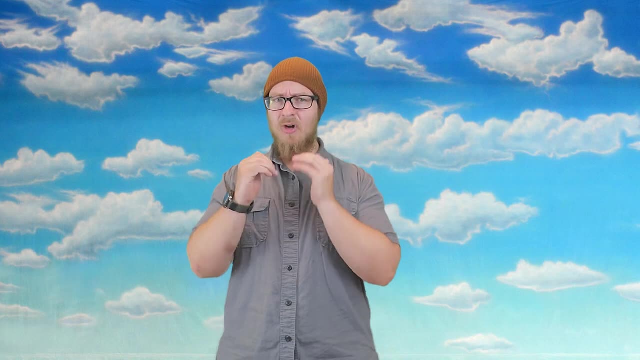 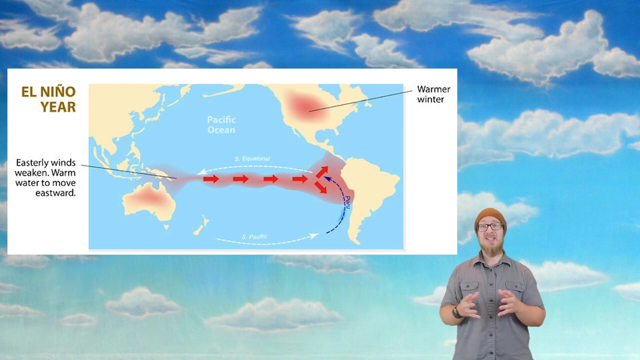 industry in South America. This does, on the other hand, produce slightly drier conditions in South America. However, sometimes the ocean temperature changes and that changes everything. The ocean-atmosphere interaction results in weaker winds, which don't push as much warm. 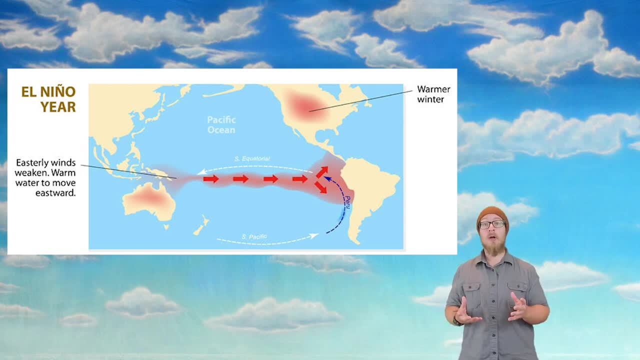 water away from South America. Well now, this warm water that is concentrated along South America causes storms there, and the reduced upwelling affects the fishing industry. Meanwhile, in the Southeast Asia side and the Australian side of the Pacific Ocean, they're experiencing much drier conditions and usually a drought. 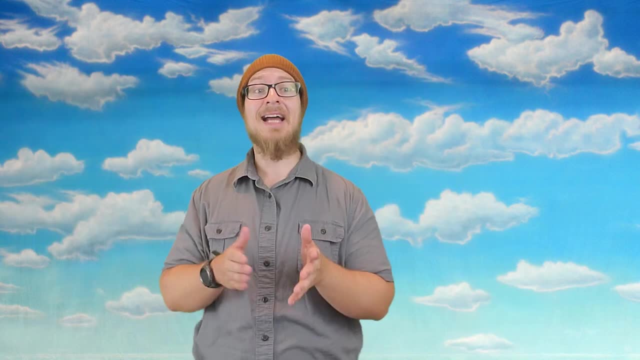 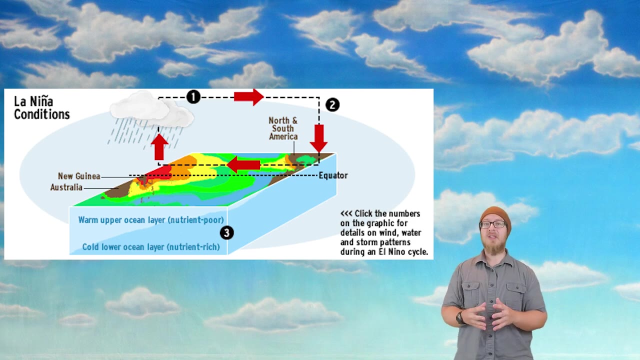 The ocean-atmosphere interaction results in weaker winds which don't push as much warm water away from South America. The opposite of an El Niño event is a La Niña event. The La Niña event is a strengthening of the normal winds which causes an exaggeration of the normal conditions. The Asia and Australia. 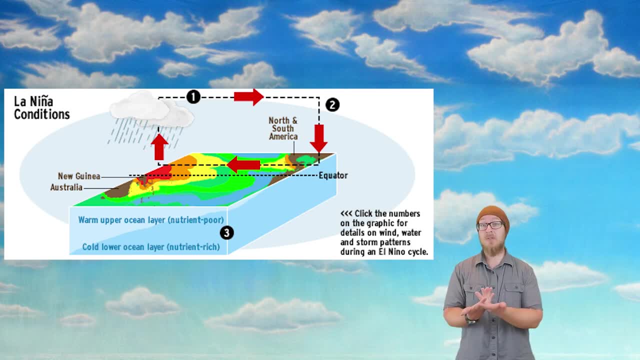 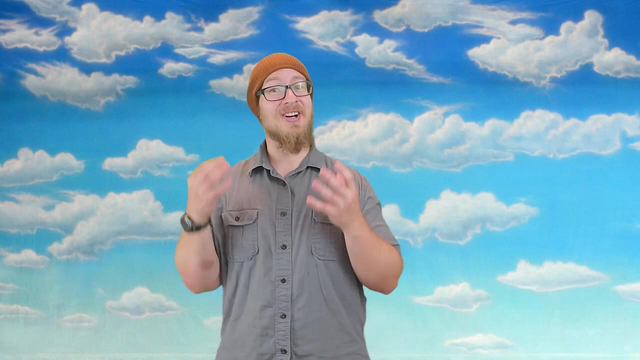 side of the Pacific Ocean sees even more rain and experience massive amounts of flooding, and the South American side may experience very dry conditions, perhaps even a drought. This wraps up our video on the atmosphere. It sure was a lot. Feel free to air your grievances. See what I did there. 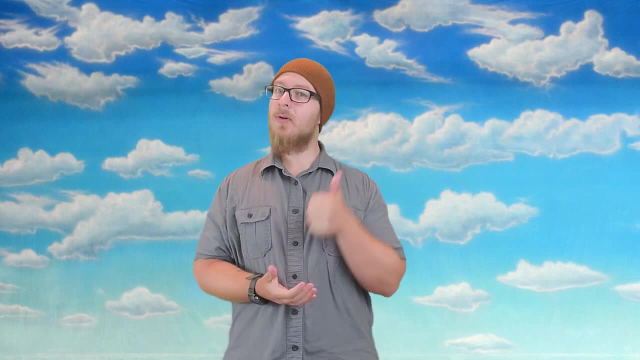 But don't air them to me. Go ahead and air them to the College Board. Thank you.